that split off early. This group is roughly divided into two families: 1., 2., 3., 4., 5., 6., 7., 8., 9., 10., 11., 12., 13.. 14., 15., 16., 17., 18., 19., 20., 21., 22., 23., 24., 25., 26., 27., 28., 29., 30.. 31., 32., 33., 34., 35., 36., 37., 38., 39., 39., 39., 40., 41., 42., 42., 43., 43.. 44., 44., 44., 44., 45., 44., 45., 46., 46., 46., 47., 47., 48., 58., 59., 52., 53.. 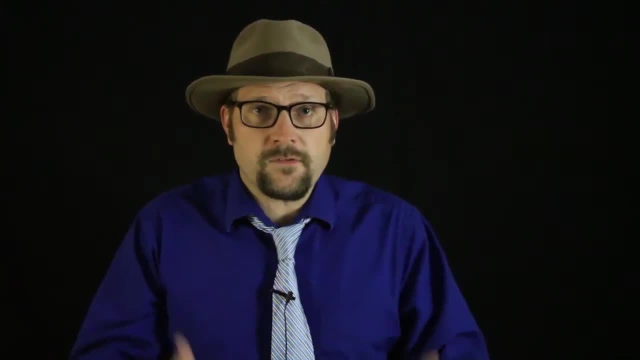 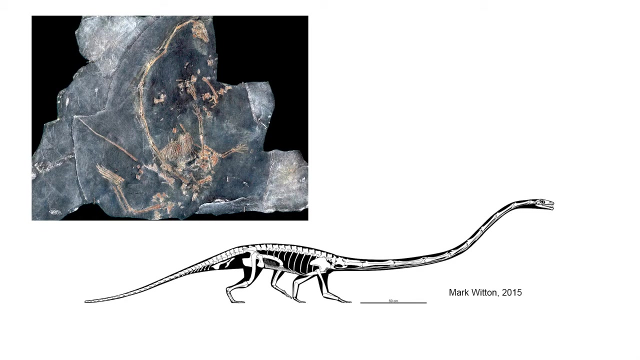 54., 55., 56., 47., 48. And the stomach contains marine cephalopods and fish supporting this theory. Yet the skeleton is not designed for a fully aquatic lifestyle, with a smaller unflattened tail, and they lack flippers in the limbs. 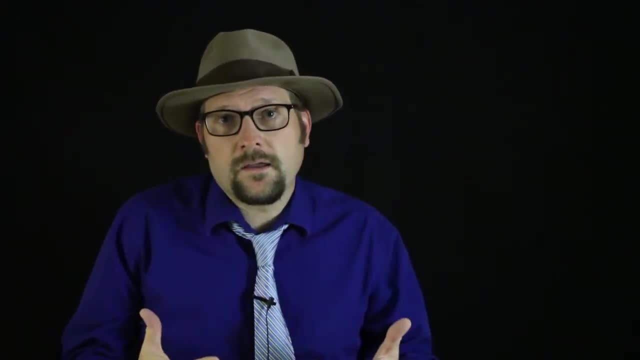 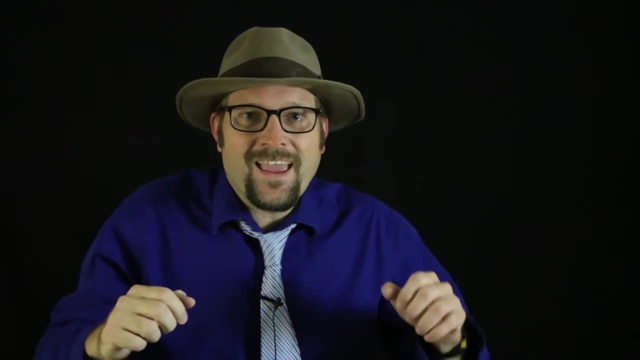 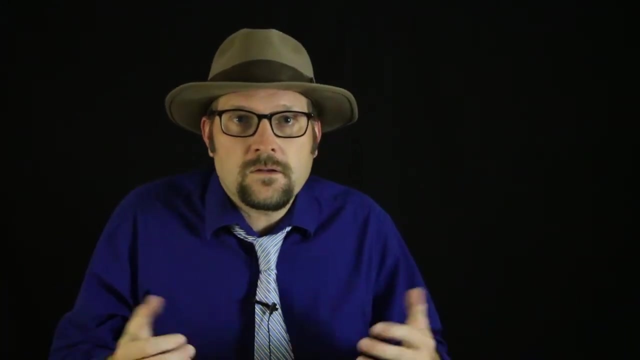 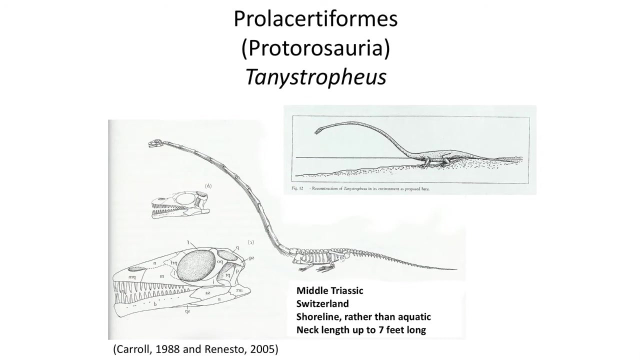 The other theory is that the animal used the long neck like a fishing pole, lowering its head over the shoreline and diving its head into the water to catch fish and other marine animals, Like a modern day herring. the long, stiff neck meant that it could reach out further. 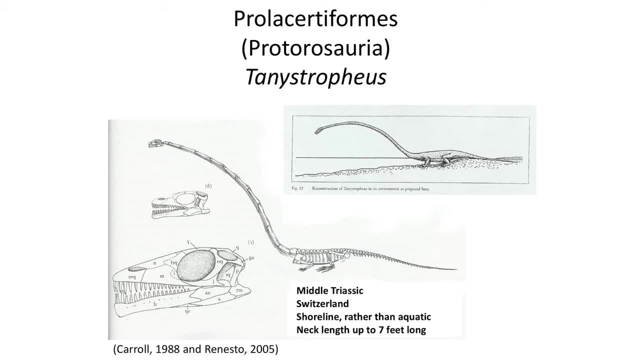 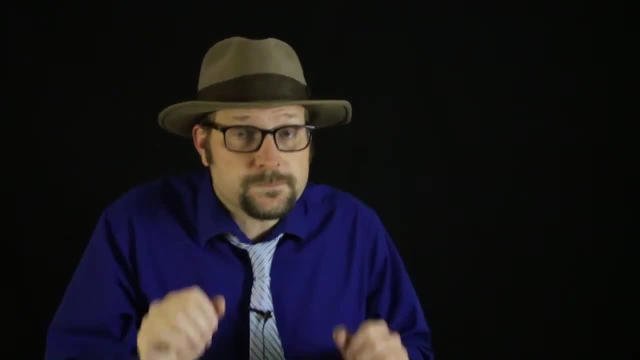 into the water to dive after prey. There would be a selective advantage to having a long neck to catch more fish. The next group of theories is that the skeleton is not designed for a fully aquatic lifestyle and that it may not be a safepical beast as well. 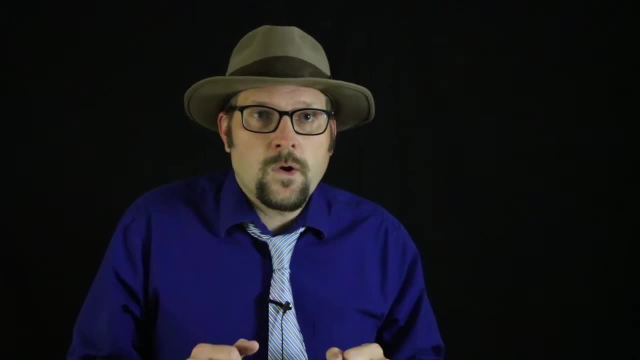 Theality directly applies that it is a very long-spinning species And obviously is not often only found by way of size, So it isn't this complex that we are seeing. Forget that they are all inuh times species and cannot be divided. 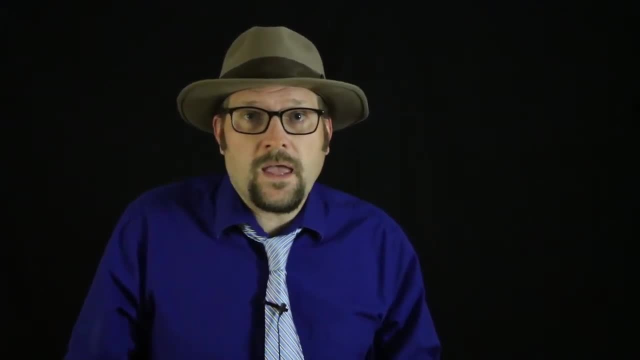 So what if the skeleton was developed? you should mark two more figures that match and eat them attached to each other. But that would probably happen one or more times and perhaps this is just the number one question we see with the fifty year of the alliance between modern Onion Epoch. 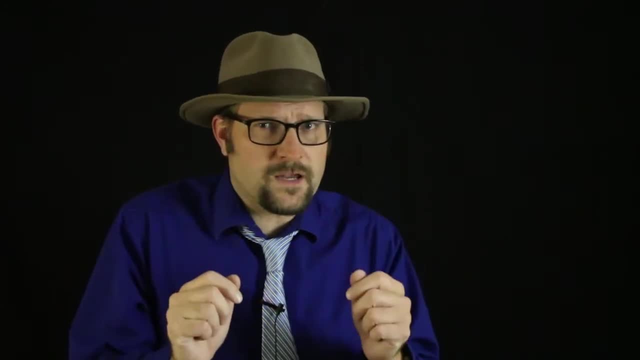 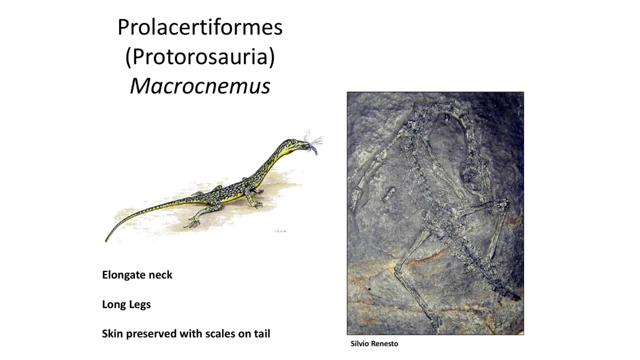 If you records an creature that has an interestingelling in your eye, Then you can't just keep doing it forever. You can forward a plan created by Abigail field as a way of contact with animals and linens. Lead did not biomass the lizard's body. 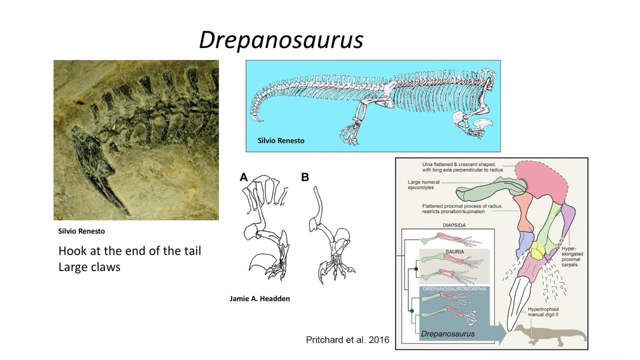 That's exactly right. you can never do that. include Drapanosaurus, which had a hook-like tail and massively large claws. It's thought that they were arboreal animals using their hook tail to hang from branches. although a recent reconstruction of the forelimb from a skeleton from the Chinle Formation in New 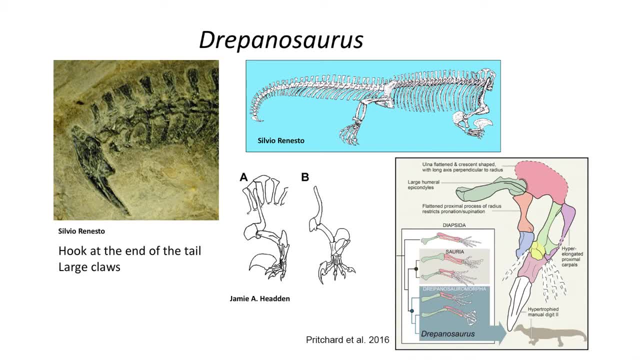 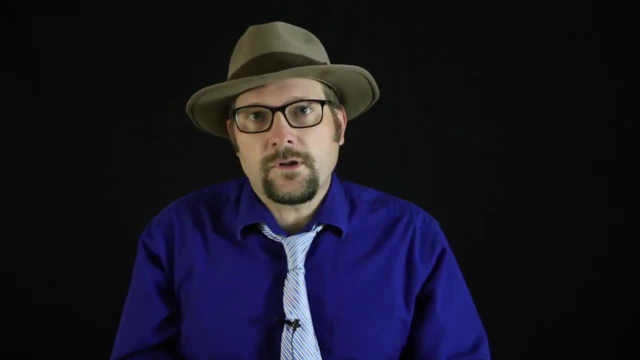 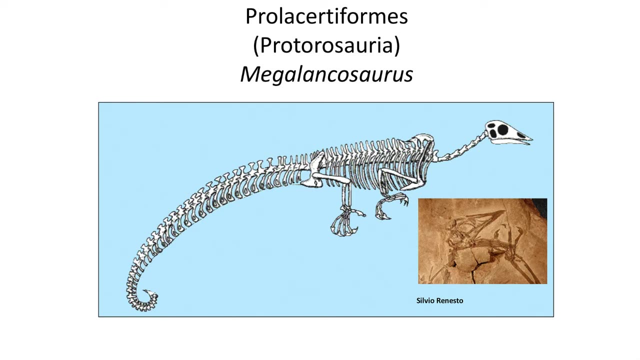 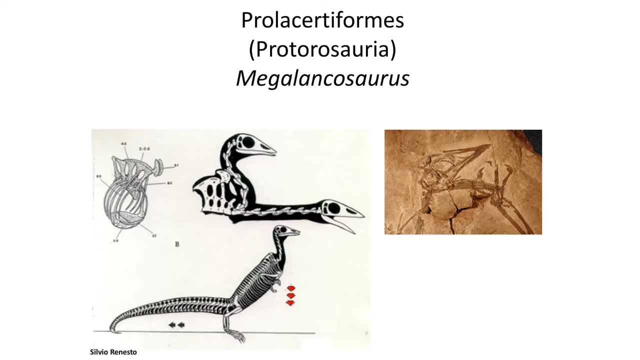 Mexico has been suggested as being highly specialized for digging using their hook-like arms. The skull of the closely related Megalachosaurus shows that it had a bird-like skull and a very stiff shoulder girdle, using its neck to possibly catch insects like modern chameleons. 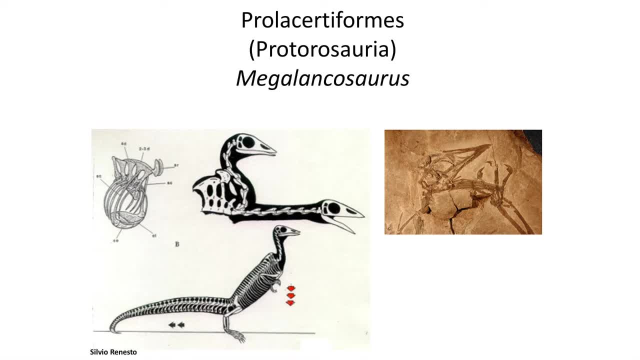 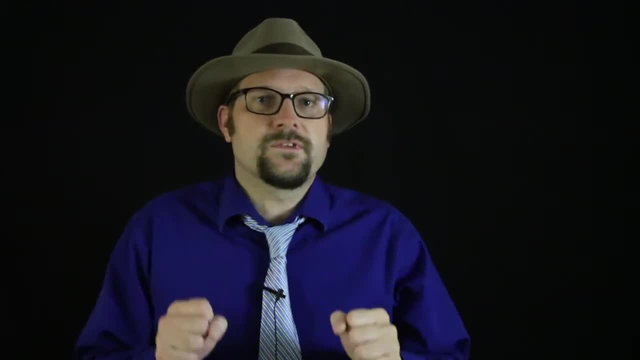 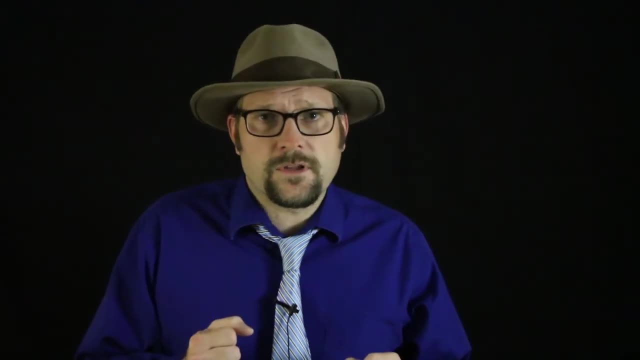 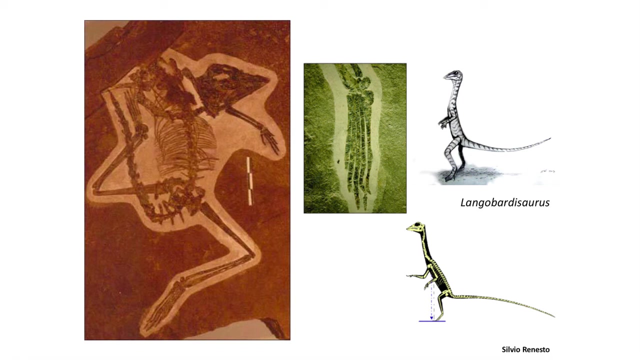 do slowly, extending the neck And able to quickly lunge to catch insect prey. The bird-like skulls and unusual skeletons have historically been involved in discussions of both bird and pterosaur origins. The well-preserved calcaneum and astragalus bones in Longbardiasaurus are distinct indicating. 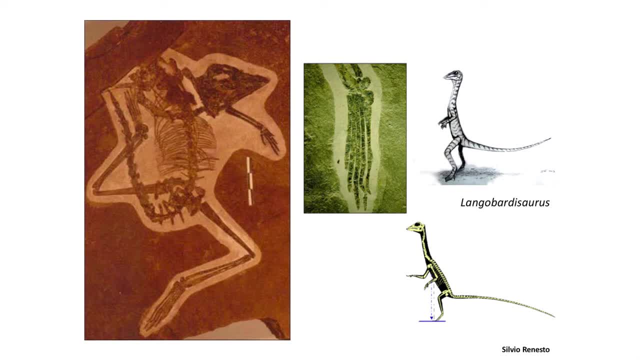 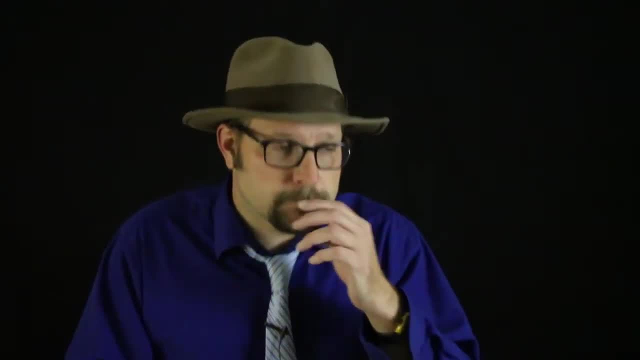 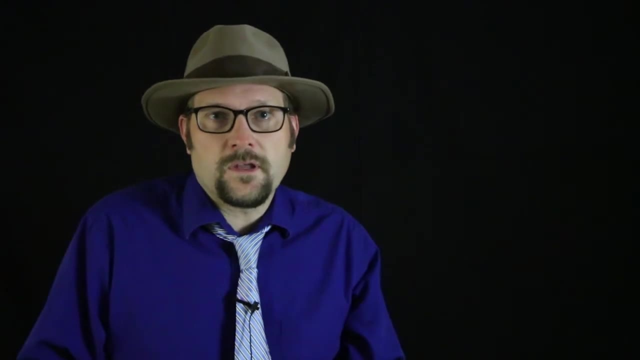 possible rotation, with the astragalus bone associated with the distal tibia But not fused with it, A primitive condition. The Prolaciformes would disappear in the late Triassic. The next group are the Trilophosauridae, a strange group of reptiles that feature peg-like. 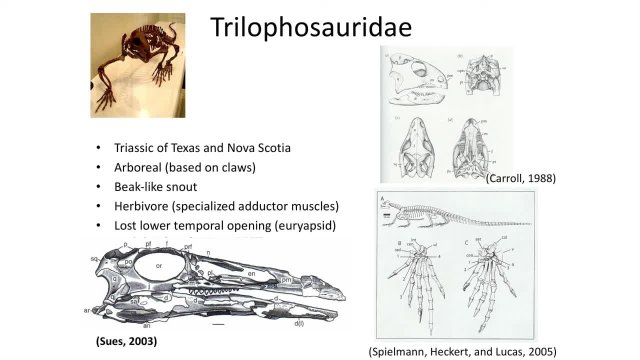 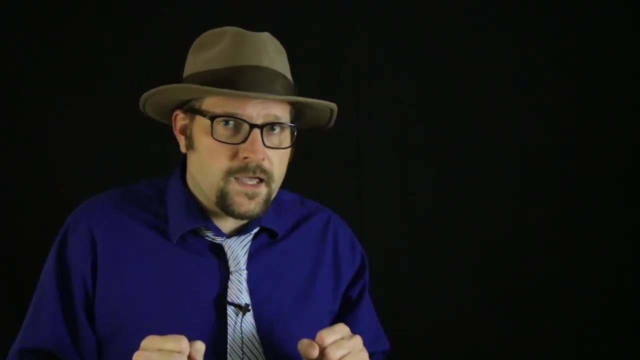 teeth, likely used for eating plants. They exhibit a uriapsid condition, with the lower temporal fenestra being lost. Primitive members have an anorbal fenestra, which is lost In some of the advanced forms. They have beak-like snouts and, based on their claws, they were likely arboreal animals living. 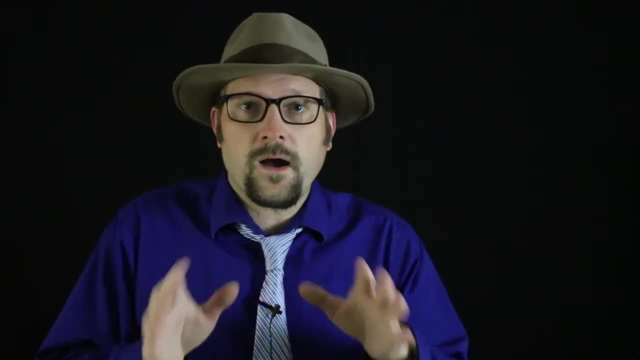 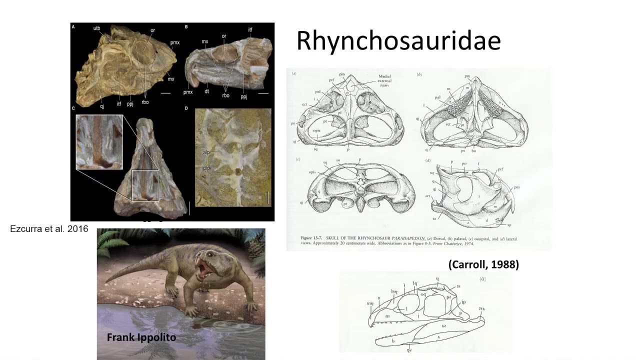 in trees. The final group are one of the more common middle to late Triassic fossils, the Rhynchosauridae, which are known from every continent except Australia and Antarctica. They have a single nostril Opening in the front of the skull. 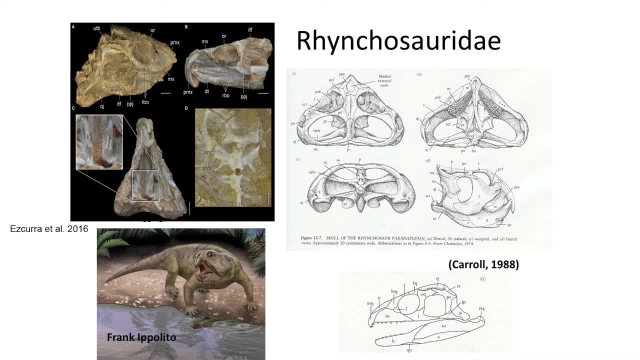 A large beak-like premaxillary bones that overlap with a hook-like denary bone to produce a strange snapping jaw. Rows of teeth on the palate but absent from the front of the mouth. The skeletons vary upright and they show adaptations for digging.